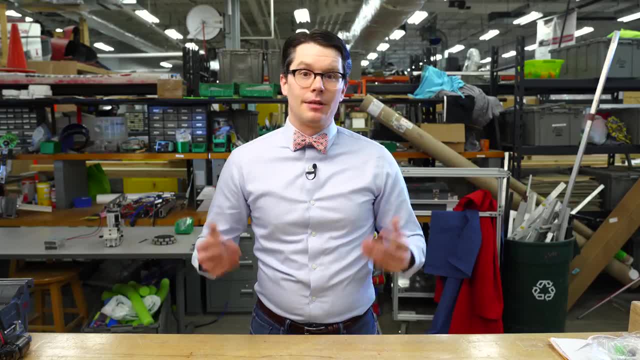 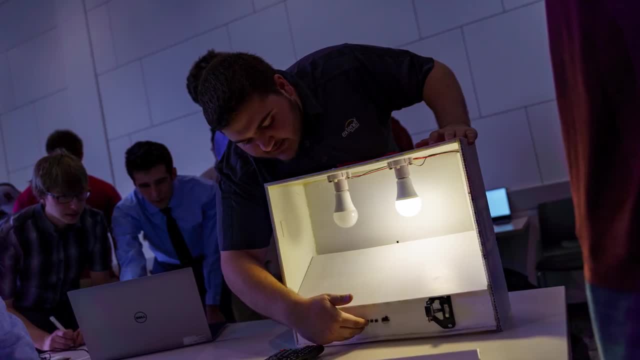 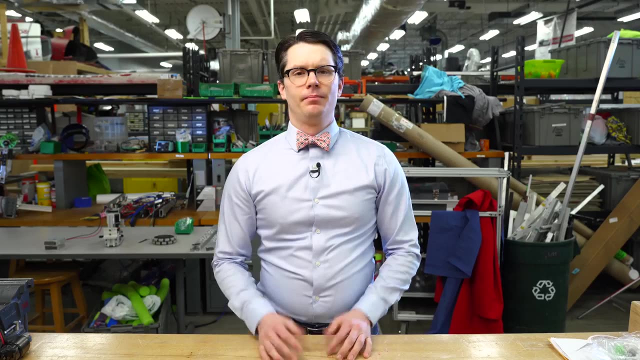 electrical engineering and computer science. In that sense, I got the best of both worlds. However, computer engineers shine in a few areas that might be difficult for either an electrical engineer or a computer scientist. These areas include embedded systems, computer architecture and digital signal processing. 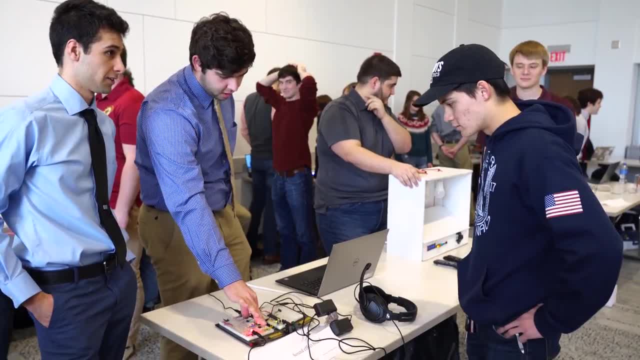 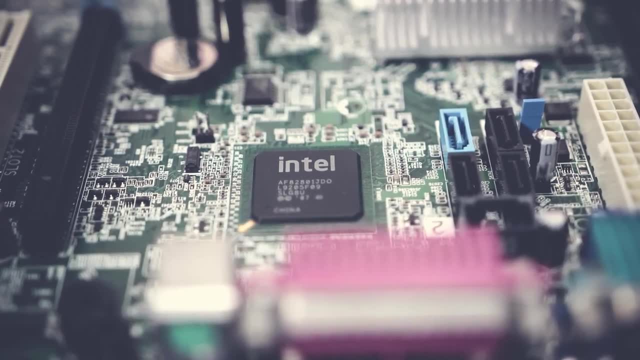 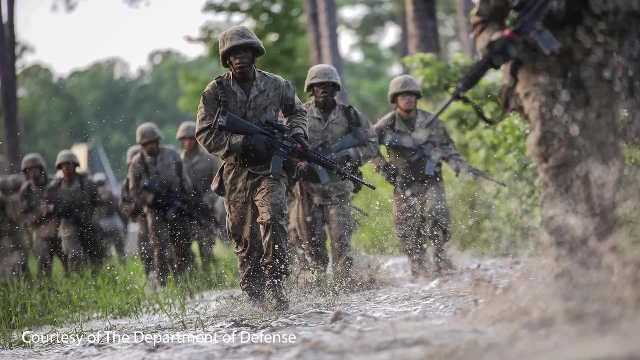 But what kind of jobs would it prepare you for? Well, you could design consumer electronics such as smartphones, smartwatches, e-book readers or maybe the next generation of Intel CPUs. Many new medical devices and scanners rely on electronics designed by computer engineers. 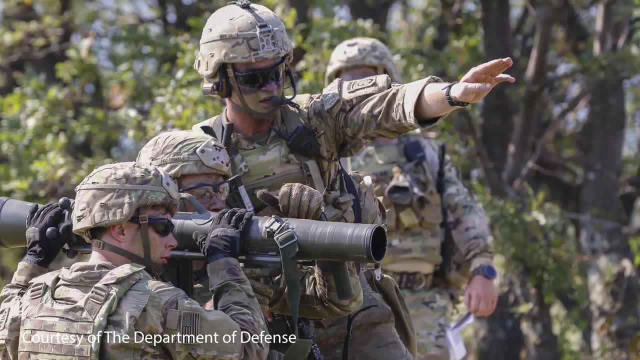 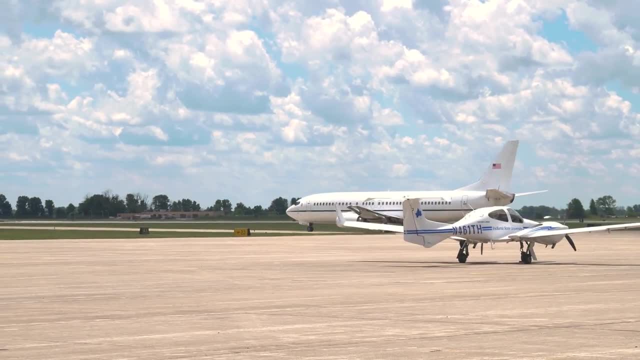 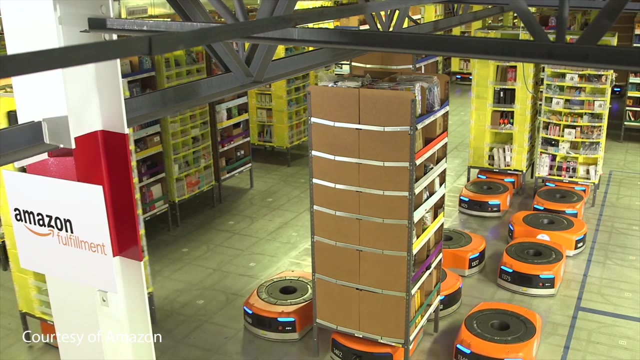 The Department of Defense and various contractors need computer engineers to create unmanned aerial vehicle flight controls and crucial satellite communication systems In aerospace. you might work on an autopilot for the next Boeing plane or create the control system for the next Mars rover. Finally, in the world of automation, computer engineers 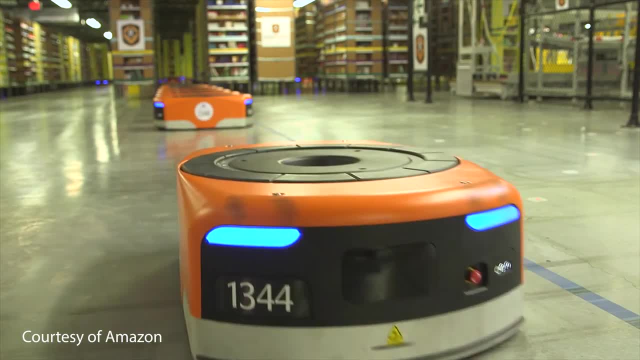 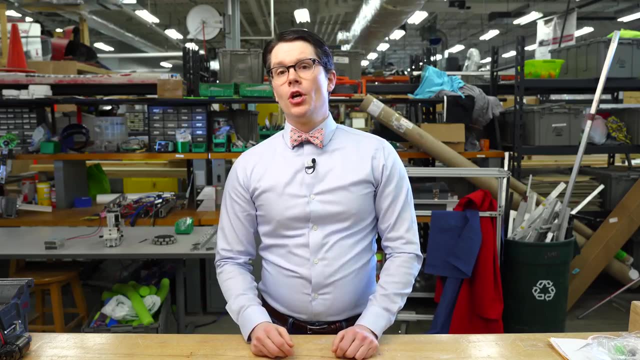 are writing low-level software for Amazon's warehouse robots that help pick and deliver goods for packaging. So what kind of classes will you take to become a computer engineer? First you'll need a healthy dose of math. Particularly you'll need calculus, differential equations and 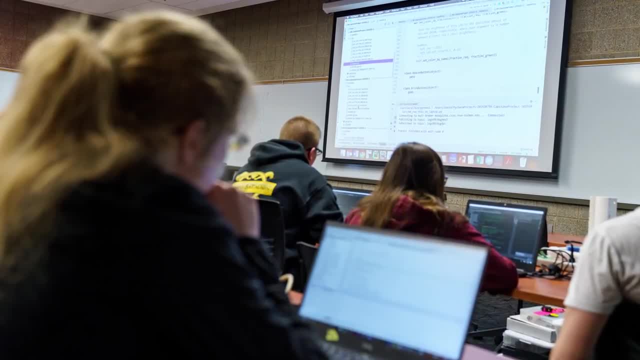 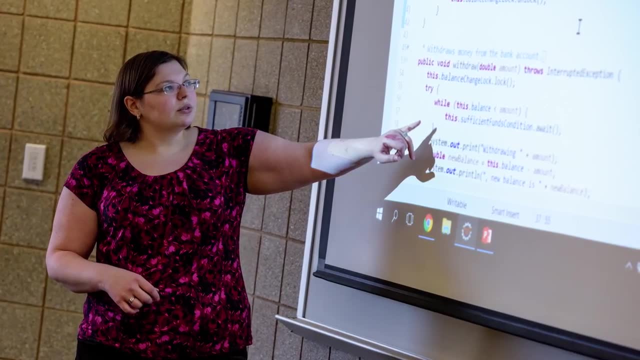 some probability theory. From the computer science side, you will likely learn a couple of programming languages. These languages allow you to write code to tell computers what to do. You might start with a low-level programming language like C to teach you the underlying concepts of how an operating system works. You might practice what you 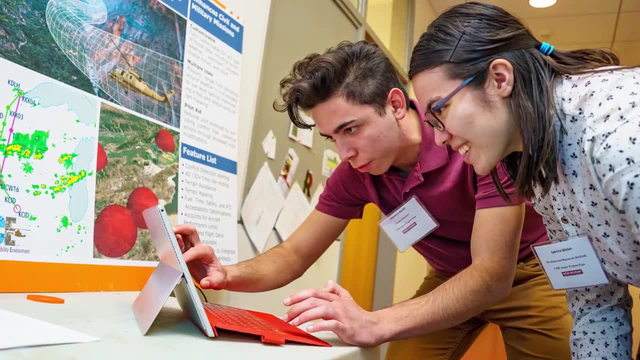 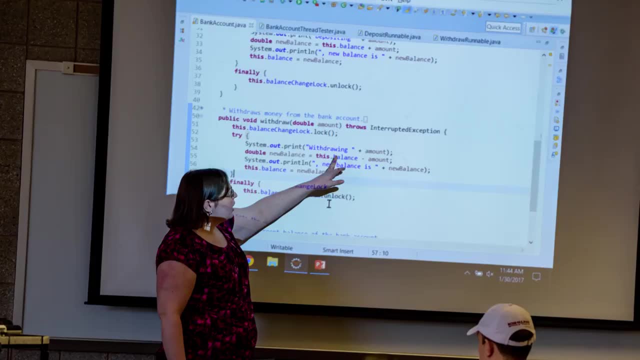 learn with a project such as writing a device driver for your computer to, say, respond to mouse clicks or read from a USB drive. You will also learn a high-level programming language such as Java or Python. These are application-level languages that teach you higher-level computer science concepts. 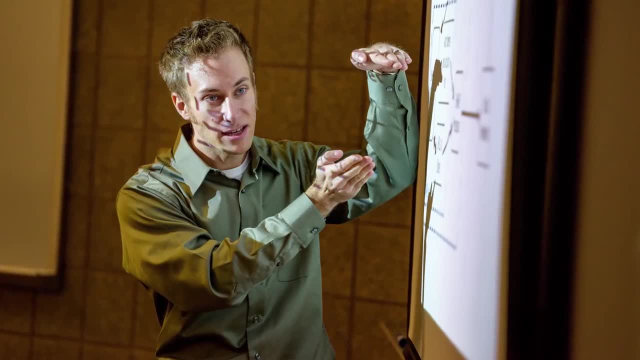 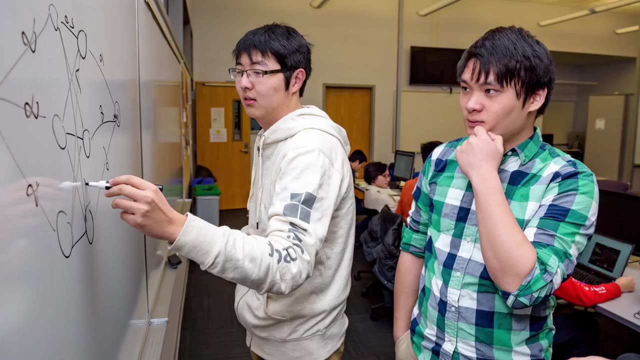 such as object-oriented programming and algorithm design. Projects might include writing a smartphone app, creating a simple game like Flappy Bird or searching through a database for customer information. You will be introduced to a variety of algorithms, which is just a fancy way of saying steps. 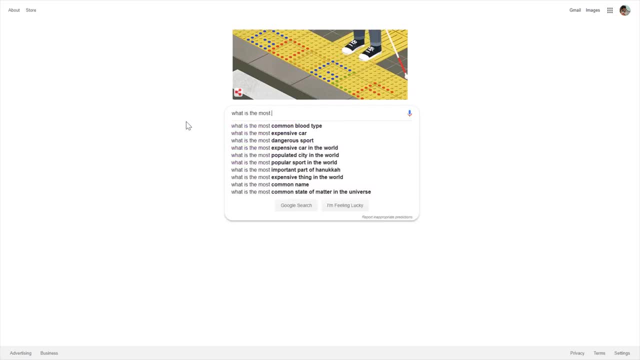 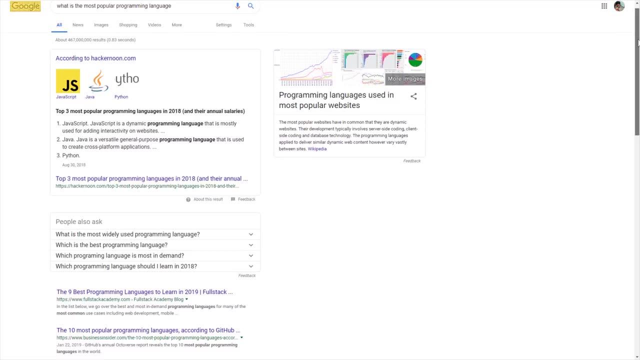 required to solve a problem. Google, for example, uses a very complicated algorithm to crawl through the internet and sort your search results, starting with the most relevant. You will learn how to develop algorithms like this and analyze them for execution time and efficiency.